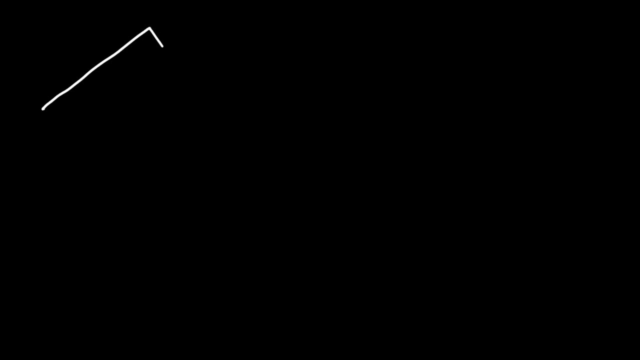 example in this problem, So I should have kept the same figure. Let's say this is A, B, C, D, E And you're given the following information: So let's say that A- B is congruent to D, C and also that angle B, A, C. 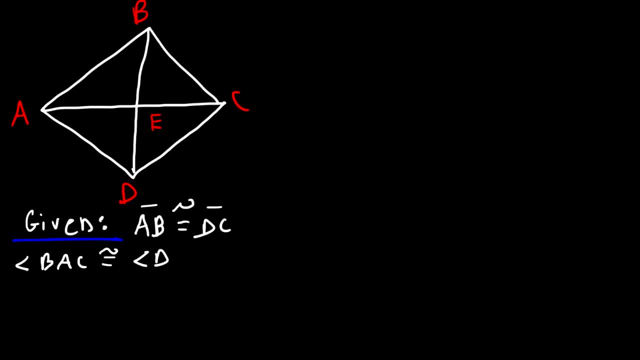 is congruent to D C A. And let's say also that angle B A, C A is congruent to D C A. And let's say also that angle B- AE is a right angle. so, with this information, go ahead and prove that the 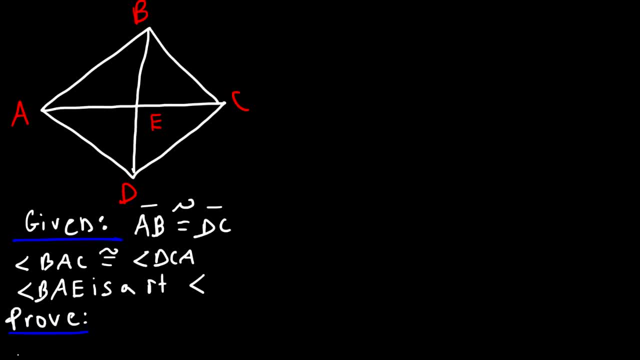 figure is a rob is so show that a, B, C, D is a rhombus. so let's start with a two column proof. so let's start with our given statement that a, B is congruent to DC. so this is given to us. we can make the following marks: so a, B is congruent to DC. now the 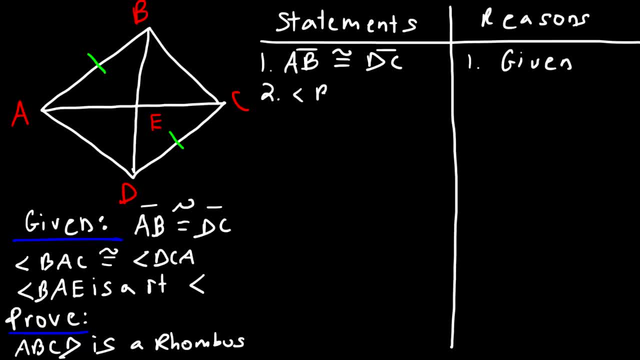 second thing that we know is that angle BAC is congruent to angle DC a, and so that's given to us as well. so this is BAC and this is DC a, so this angle is congruent to that angle. now we know that these two angles are congruent. 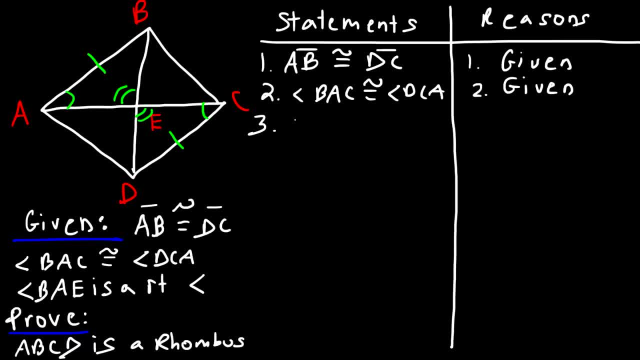 to each other. they form vertical angles. so we could say that angle a, e, B is congruent to angle C, e, D and the reason: the vertical angle theorem. we could say that vertical angles are congruent. so now we can prove that these two triangles are congruent. so let's say that triangle. 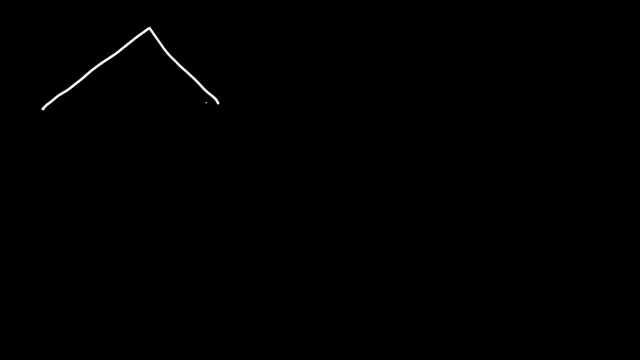 in this problem, So I should have kept the same figure. let's say this is abcde And you're given the following information: So let's say that AB is congruent to DC And also that angle, BAC is congruent to DCA. 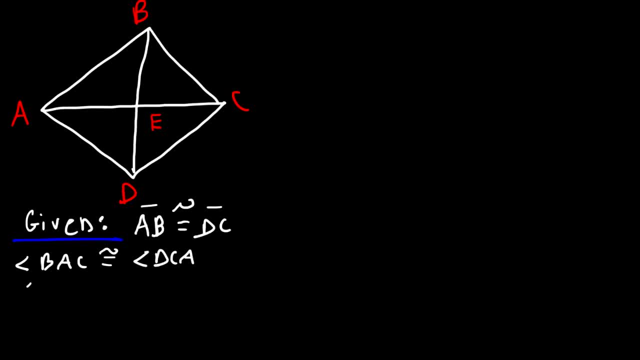 And let's say also: angle BAE is a right angle. So with this information, go ahead and prove that the figure is a rhombus. So show that ABCD is a rhombus. So let's start with a two-column proof. 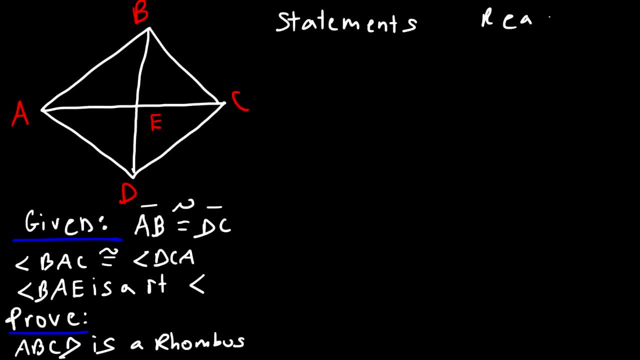 So let's start with our given statement that AB is congruent to DC. So this is given to us And we can make the following marks: So AB is congruent to DC. Now the second thing that we know is that angle BAC. 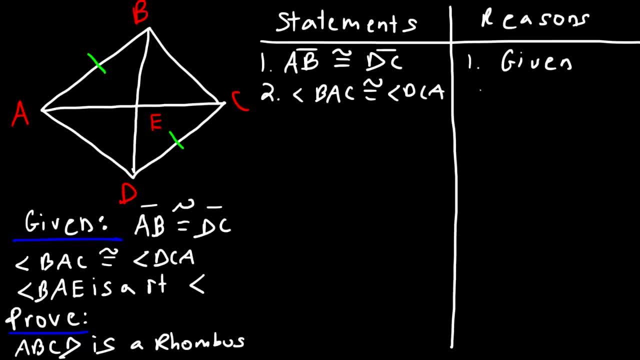 Is congruent to angle DCA And so that's given to us as well. So this is BAC And this is DCA, So this angle is congruent to that angle. Now we know that these two angles are congruent to each other. 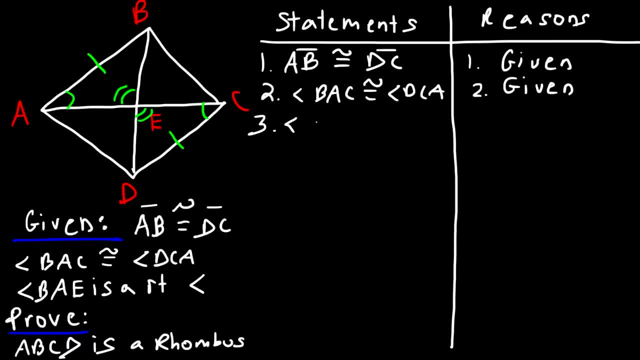 They form vertical angles. So we could say that angle AEB is congruent to angle CED. And the reason? the vertical angle theorem. We could say that vertical angles are congruent. So now we can prove that these two triangles are congruent. 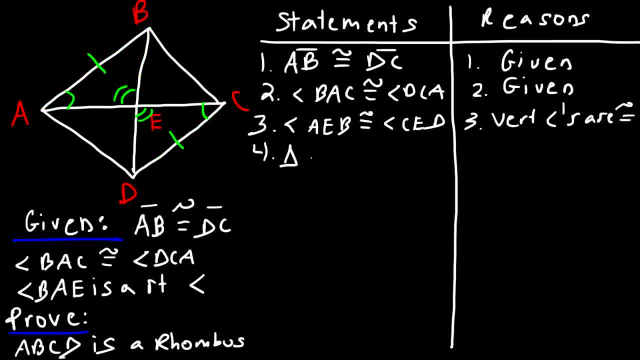 So let's say that triangle AEB is congruent to triangle CED, And the reason for this? It's the angle angle side postulate, And this is based on statements 3,, 2, and 1.. So now that we've shown that, 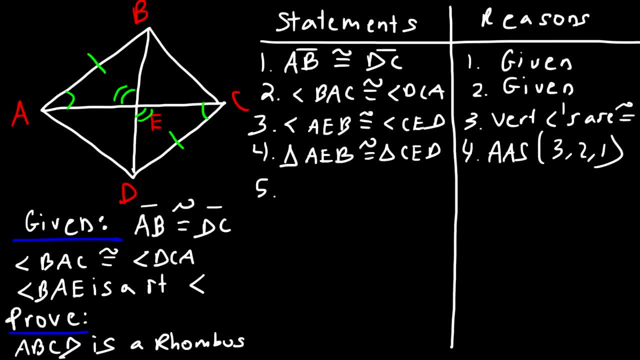 Those two triangles are congruent, Their corresponding parts must be congruent as well. So therefore we could say that AE and EC are congruent, And this is based on CPC, CPC, TC. There we go. Now we could also say: 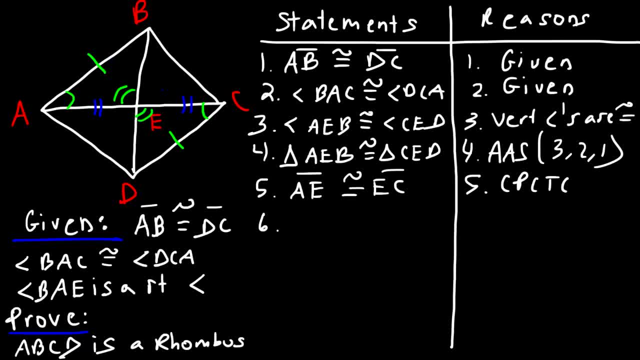 Let's use two marks to distinguish it from that one. We could say that BE is congruent to ED, Because there's still part of this, The two triangles that we've proven to be congruent, And this is also due to. 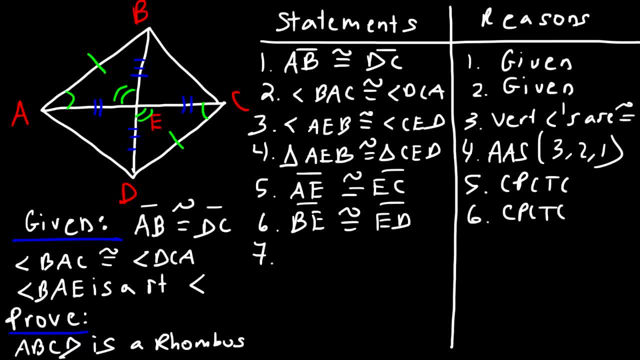 CPC TC. So now step 7.. What else can we say Now? keep in mind That we also have this given statement. Angle BAE Is a right angle And that's given to us, So that means this is a 90 degree angle. 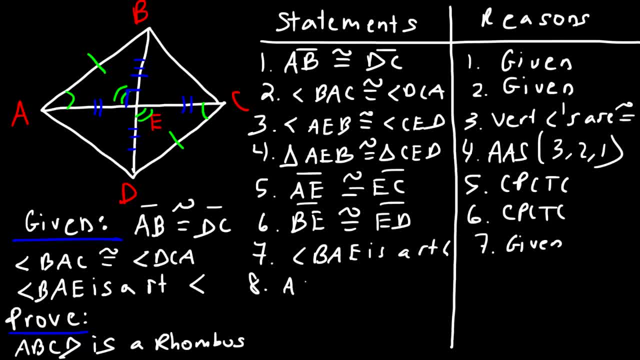 So now we can also say that AC Is the perpendicular bisector Of BD. As you can see, AC Splits BD into two equal parts And it meets BD at a right angle. And also BD Does the same thing for AC. 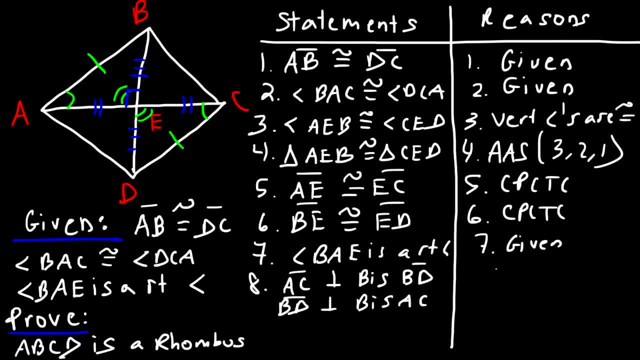 It's the perpendicular bisector of AC, And so I'm going to write Definition Of A perpendicular bisector. So now that we've shown That the diagonals They bisect each other at right angles, Now we can make the statement that 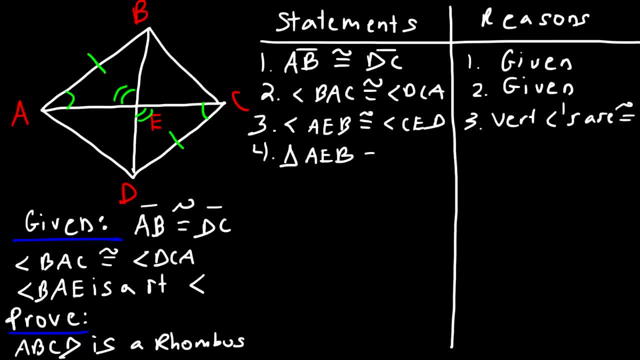 AEB is congruent to triangle CED and the reason for this? it's the angle angle side postulate, and this is based on statements 3, 2, & 1. so now that we've shown that those two triangles are congruent, their corresponding parts must be congruent as well. 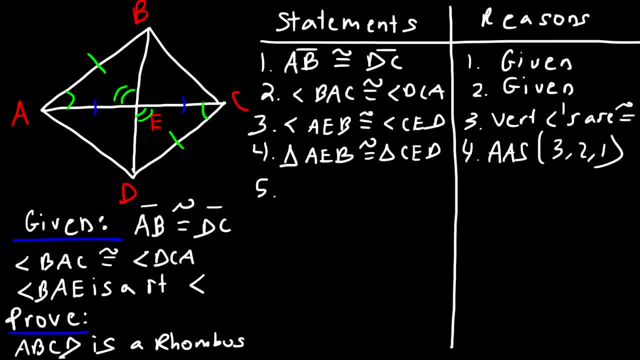 So, therefore, we could say that AE and EC are congruent, And this is based on C-P-C-C, C-P-C-T-C. There we go. Now we could also say: let's use two marks to distinguish it from that one. 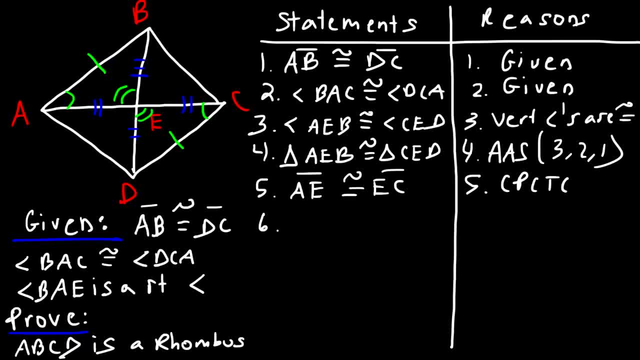 We could say that BE is congruent to ED, because they're still part of this, the two triangles that we've proven to be congruent, And this is also due to C-P-C-T-C. So now step seven. What else can we say? 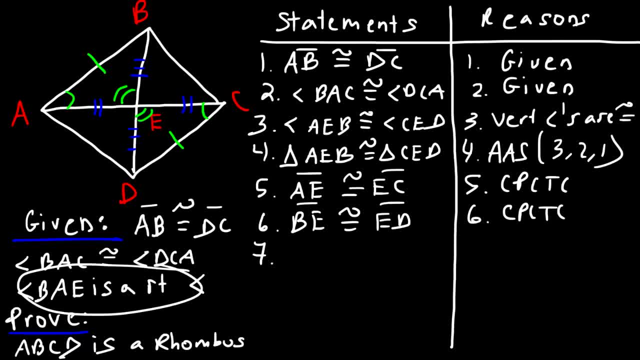 Now keep in mind that we also have this given statement. Angle BAE is a right angle And that's given to us. So that means this is a 90 degree angle. So now we can also say that AC is the perpendicular bisector of BD. 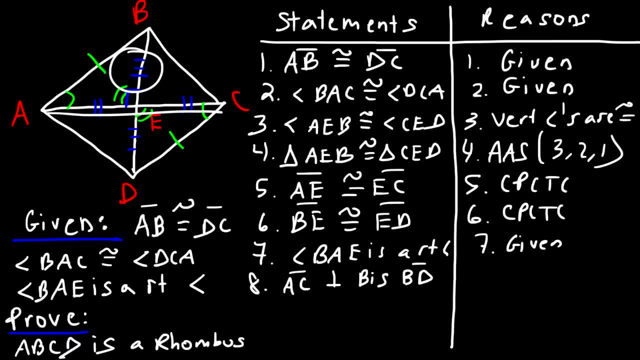 As you can see, AC splits BD into two equal parts And it meets BD at a right angle. And also BD does the same thing for AC. It's the perpendicular bisector of AC, And so I'm going to write definition of a perpendicular bisector. 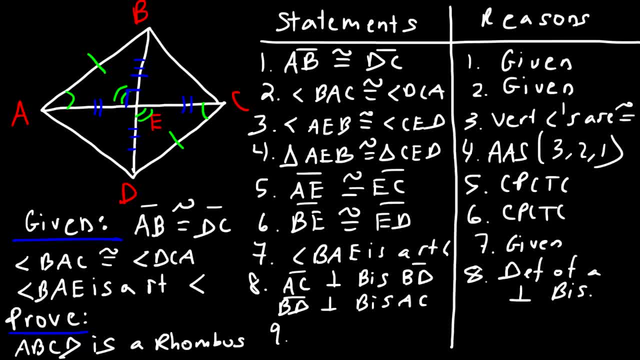 So now that we've shown that the diagonals, they bisect each other at right angles, Now we can make the statement that ABCD is a rhombus. Now we can make the statement that ABCD is a rhombus. Now we can make the statement that ABCD is a rhombus. 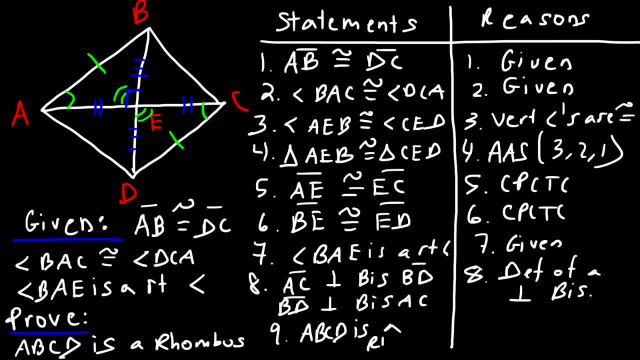 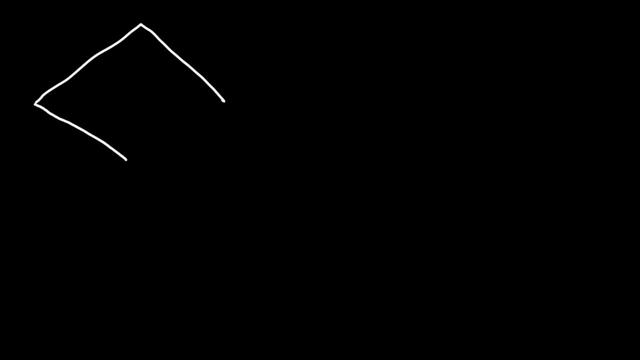 ABCD Is a rhombus And for the reason I'm going to write Definition Of A rhombus. Now let's work on another example. Let's prove that this figure Is a rhombus. So here's what we're given. 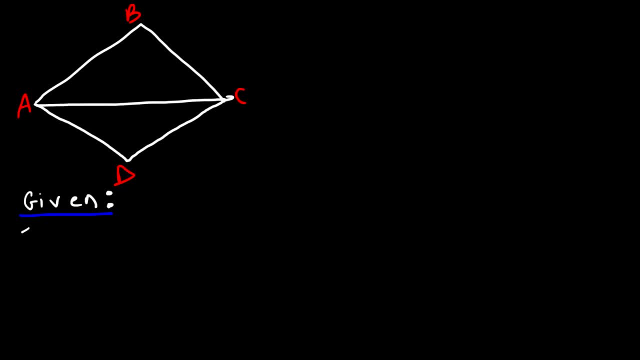 We're given that angle A Is congruent To angle C And also that angle B Is congruent to angle D, And we're also told that Angle BAC Is congruent To angle BCA. So, with this information, 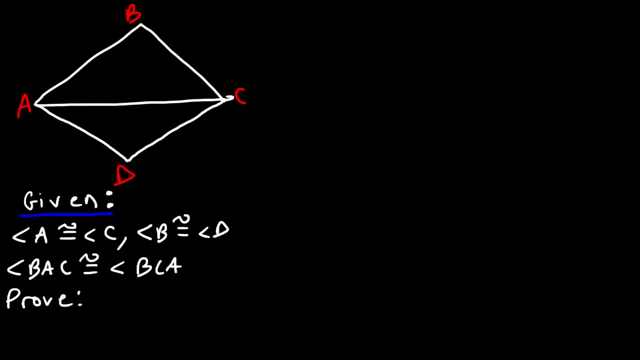 Prove That ABCD Is a rhombus Is A rhombus, Or if we see That the rhombuses Is a rhombus, Is, If Located, So in any scenario That angle. 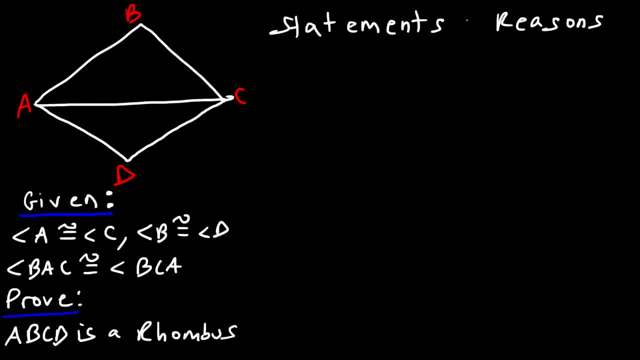 Is congruent To angle A. We'd want to know what position The rhombus Is. Is About The position Of Its Zone Or angle SHM? Let's sinking. That'll actually Hypothetically. 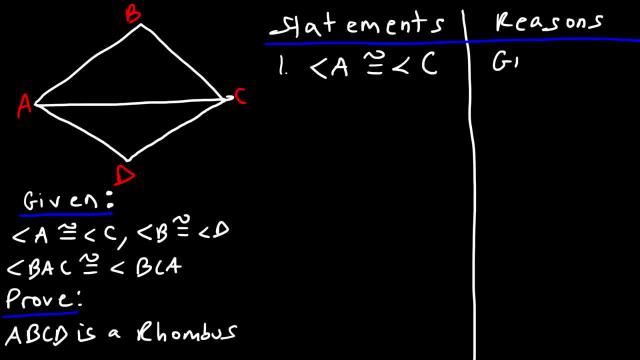 Hypothetically, And that angle would shift Out To the same point. So That means At Location That people Sitting Music Using. so this is angle a, that's angle C. number two, angle B, is congruent to angle D and 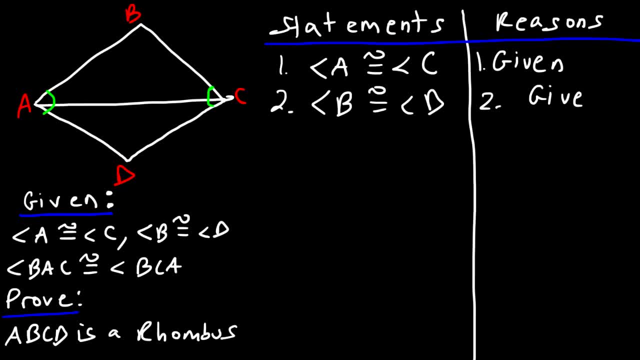 that's also a given statement, so we can mark that here. so notice that the opposite angles are congruent. so therefore we can say that a, B, C, D is a parallelogram. if the opposite angles are congruent, then we have a parallelogram. so we can write definition of a parallelogram. or you can say if 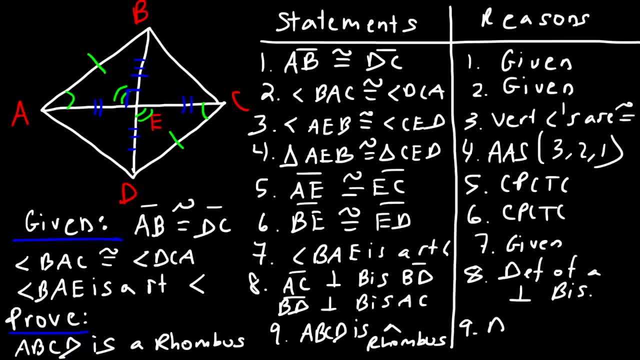 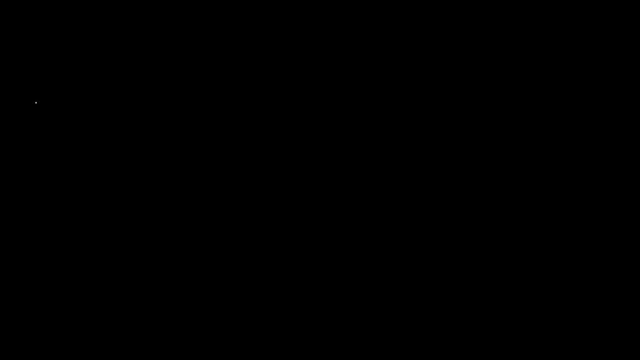 And for the reason I'm going to write definition of a rhombus. And for the reason I'm going to write definition of a rhombus, Now let's work on another example. Now let's work on another example. Let's prove that this figure is a rhombus. 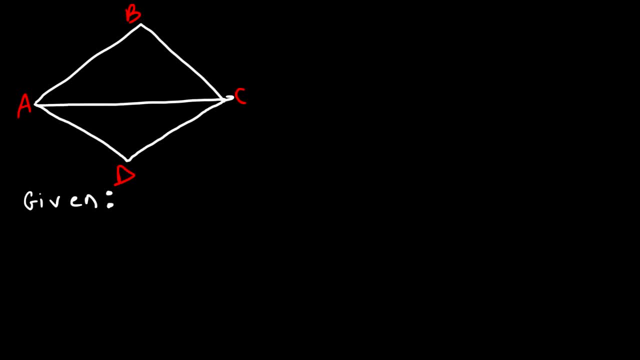 So here's what we're given. So here's what we're given. We're given that angle A is congruent to angle C, and also that angle B is congruent to angle D, And we're also told that angle BAC is congruent to angle BCA. 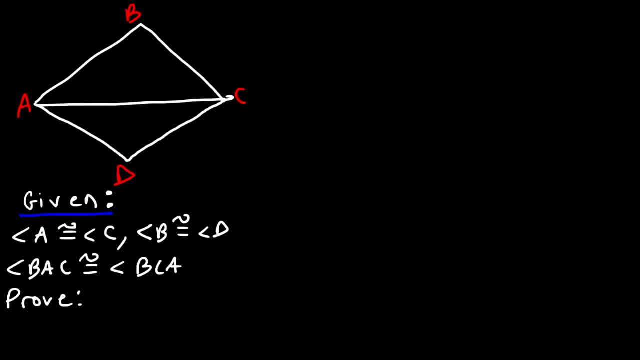 So would this information prove that ABCD is a rhombus? So let's start with the information that we're given. Okay, So, number one: we know that angle A is congruent to angle C, and that's given to us. 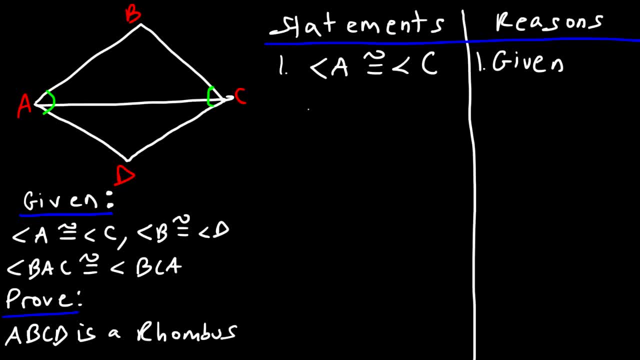 So this is angle A, that's angle C. Number two, angle B, is congruent to angle D, and that's also a given statement, So we can mark that here. Okay, So notice that the opposite angles are congruent. So therefore we can say that ABCD is a parallelogram. 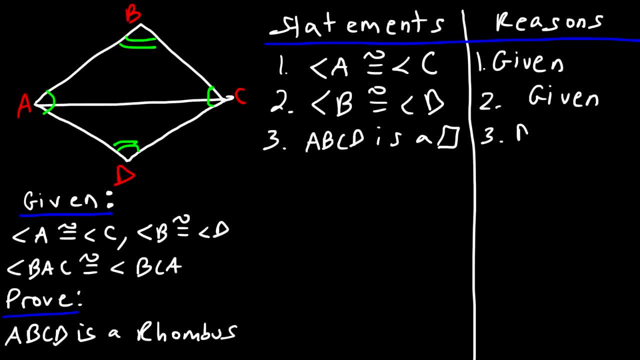 If the opposite angles are congruent, then we have a parallelogram. So we can write definition of a parallelogram or we can say: if opposite angles are congruent, then the quadrilateral is a parallelogram. Now let's move on to our next given statement, and that's angle. BAC is congruent to angle.